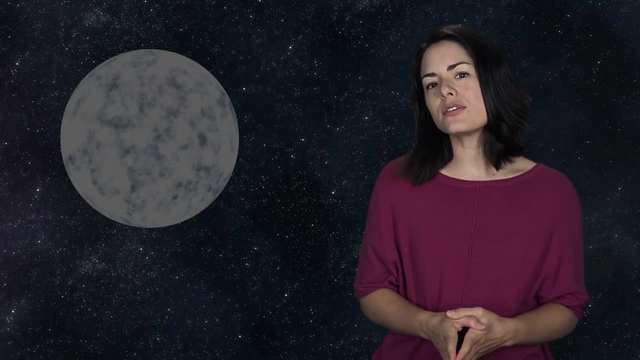 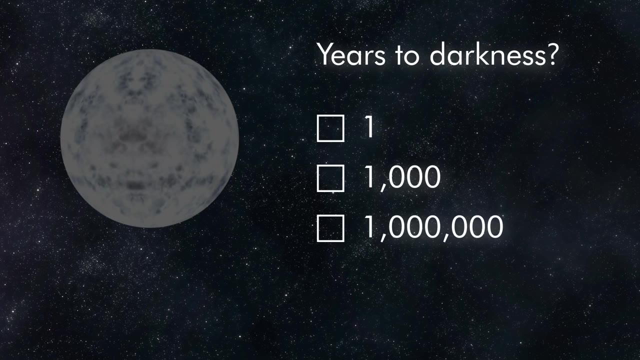 cold, close to absolute zero. So how long do you think it will take the white dwarf to cool down to the point that it goes dark? One year, A thousand years? A million years? It's believed it will take trillions of years for white dwarfs to stop glowing. That's. 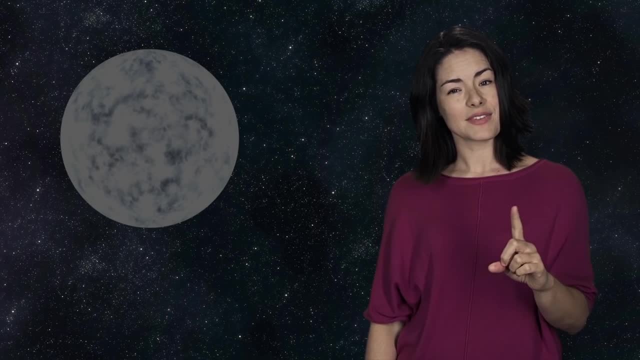 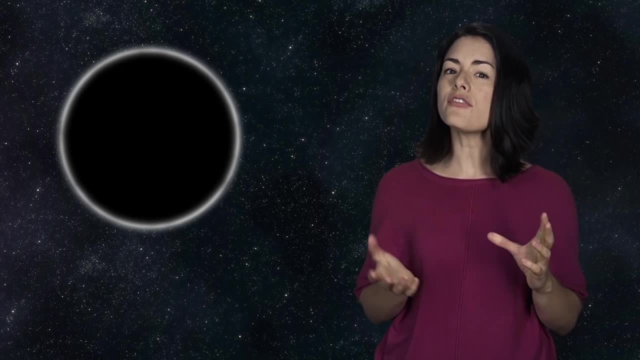 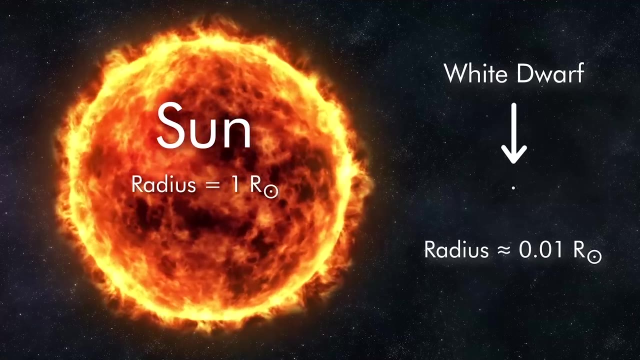 But one day we'll find out. Somewhere in space the lights will go out in a white dwarf. At that point, all that's left is a dead ball of dark matter, which we call a black dwarf. Although white dwarfs are small compared to burning stars, they're still quite massive. 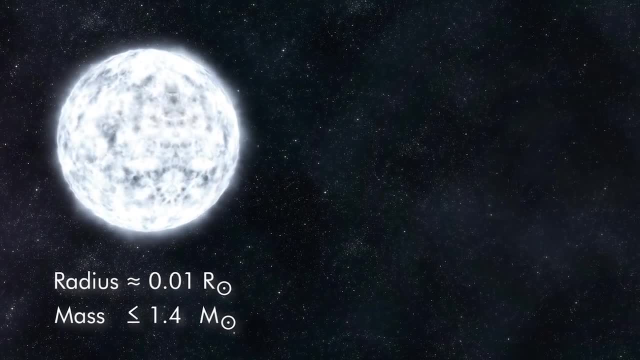 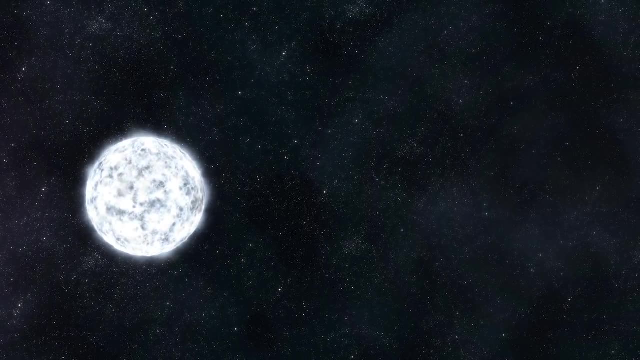 Their mass can be as high as 1.4 solar masses, a value called the Chandrasekhar limit. Because of their large mass, gravity very tightly compresses the stellar matter, But at some point you run up against the Pauli exclusion principle. 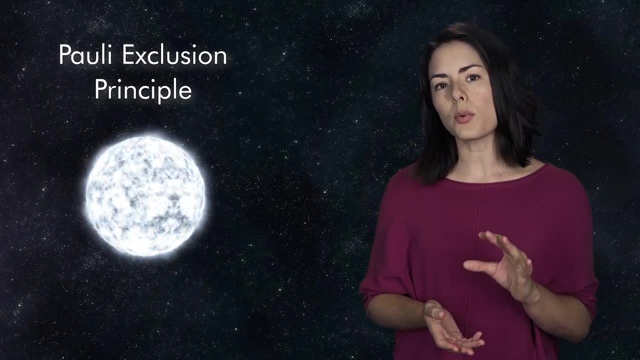 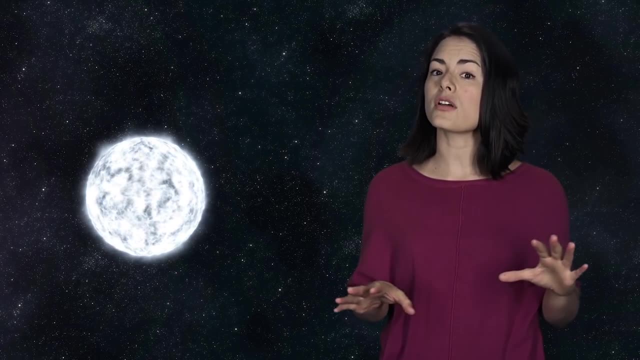 This idea from quantum mechanics says basically that two identical particles cannot occupy the same place at the same time. For white dwarfs, the pressure from gravity has stripped all the electrons from the atoms. Gravity then packs the electrons so closely together that the Pauli exclusion principle 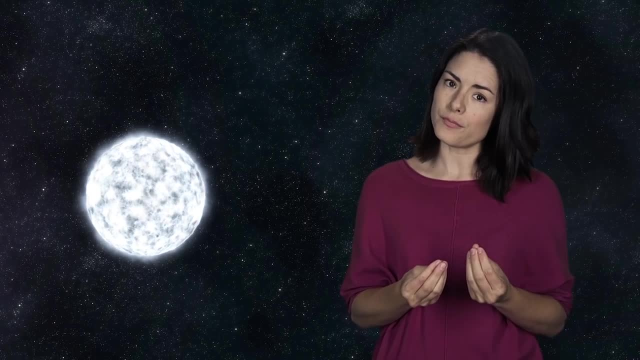 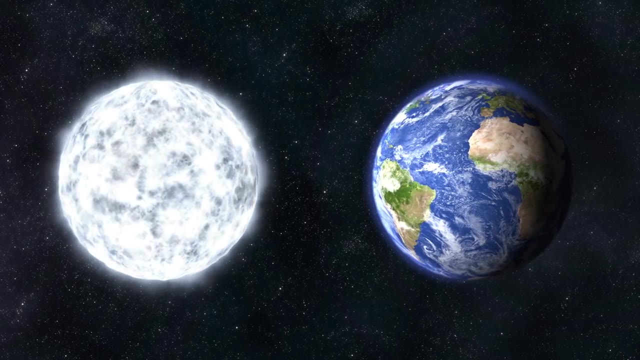 kicks in and stops the white dwarf from shrinking any further. This is called the degenerate electron pressure. White dwarfs are about the size of an Earth-like planet and shine with only a fraction of the brightness of a star. So how do you find and observe them? 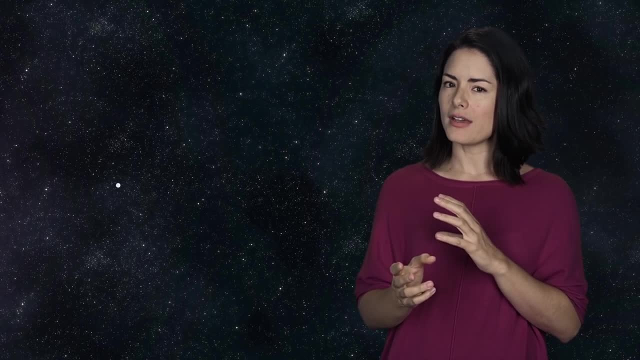 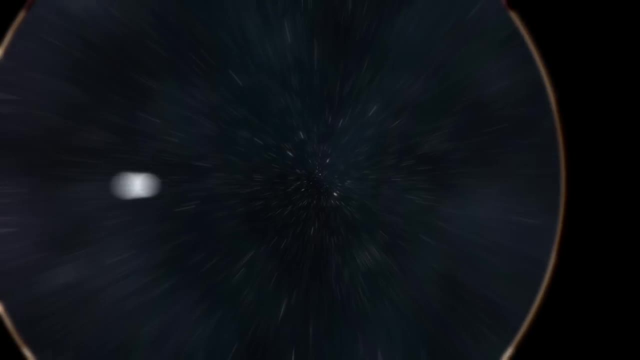 One way is to look for stars with an unexplained back-and-forth motion. This suggests a massive companion. If you can't see the companion, it's probably a black hole, But oftentimes telescopes are able to see a small, dim neighbor, a white dwarf. 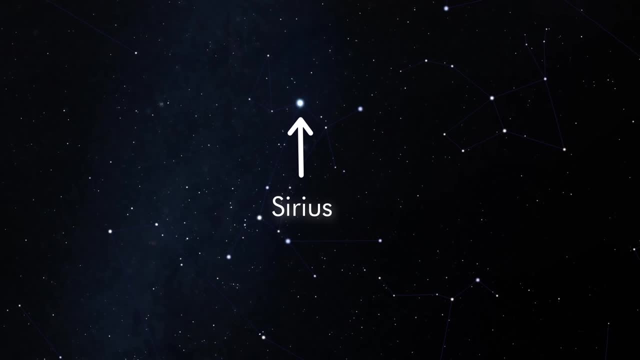 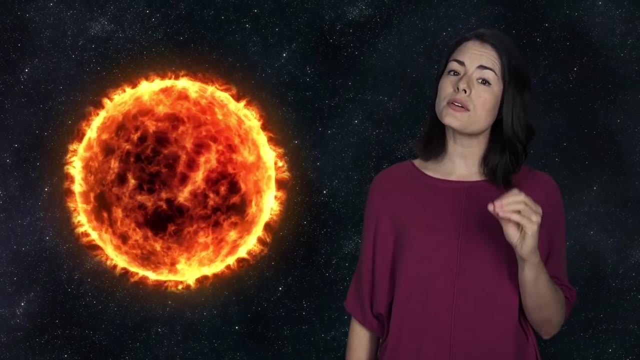 In fact the brightest star in the night sky, Sirius, has a white dwarf companion, which we call Sirius B. There's another way to find white dwarfs, And it's due to a curious phenomenon which occurs near the end for some stars. 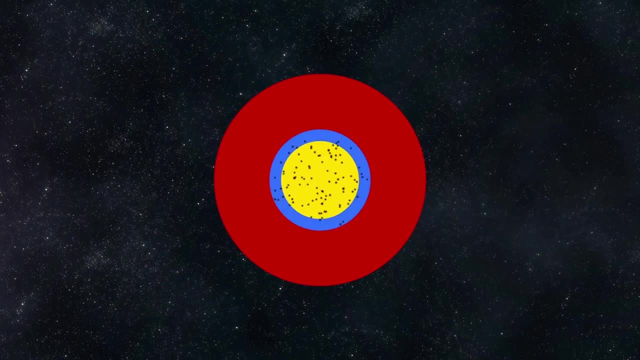 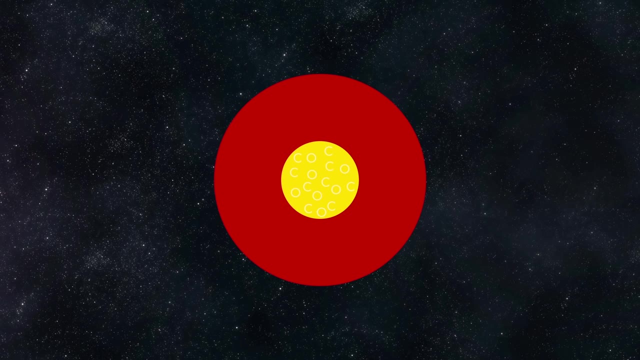 Earlier we mentioned that fusion can occur not just in the core but in the shells around the core. When a star begins to die, fusion may stop in the core. That's because the core is now made of heavier elements and there isn't a strong enough.